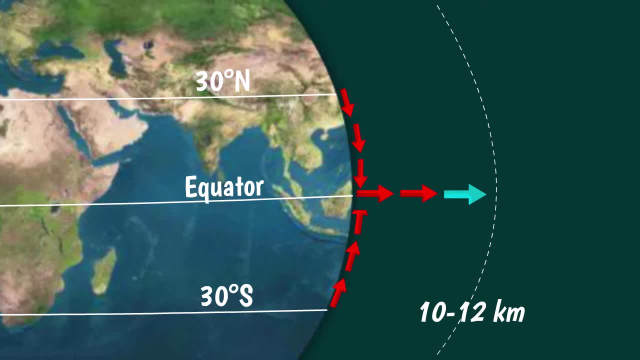 it cannot rise any further. Pushed from below by the air, which continues to rise, but blocked in its ascent, the air aloft begins to move towards the poles and when it arrives at a latitude of about 30 degrees, the air will begin to move towards the poles and when it arrives at a 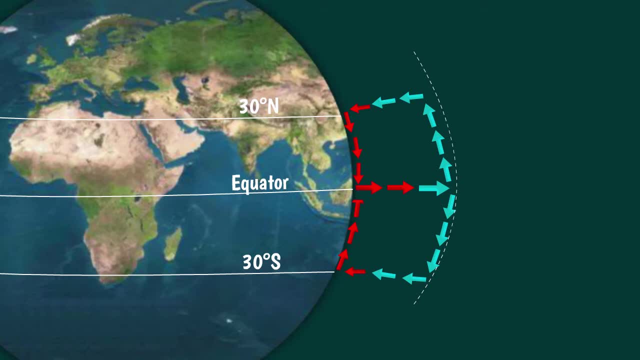 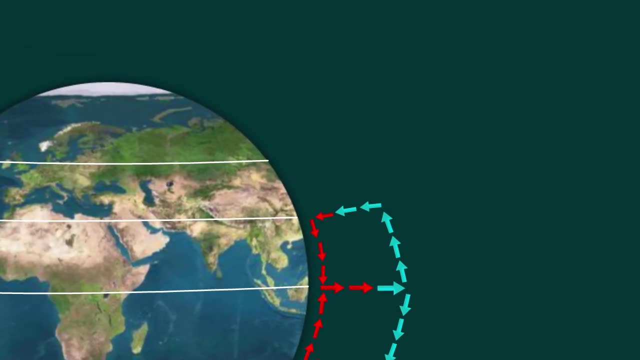 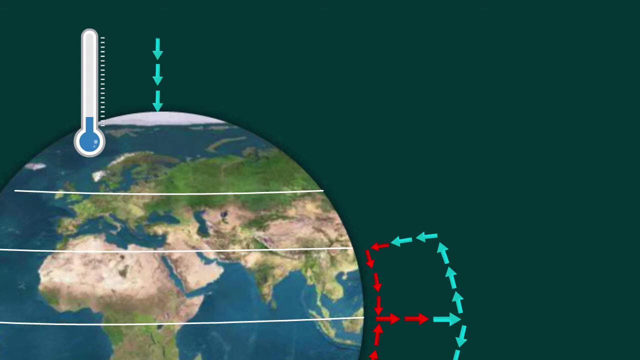 low altitude, it falls back to the surface. This completes a loop called the Hadley cell, from the scientist who first described it. A similar loop exists above the poles. Indeed, when the air cools, it becomes heavier and pushes against the surface of the earth Along. 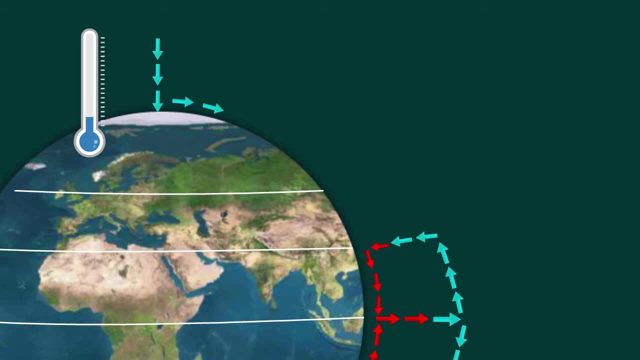 the surface. the air is therefore forced to slide to lower latitudes. On the contrary, at altitude, the air is drawn towards the poles. This cell, called polar cell, is completed by a loop located at a latitude of about 50 degrees, above which air rises. Now let us see what. 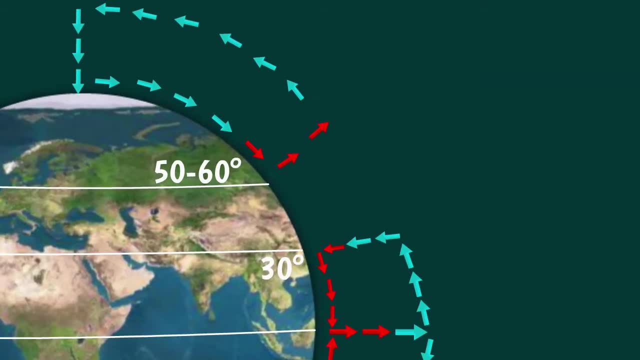 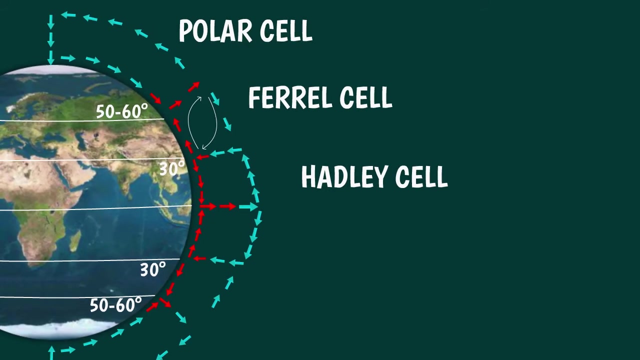 happens between 30 degrees and 50 degrees latitude, As we have seen, when the air rises or falls, it is replaced by air coming from the sides. This creates a third cell, the ferrule cell, which differs from the other two because it spins in the opposite direction. 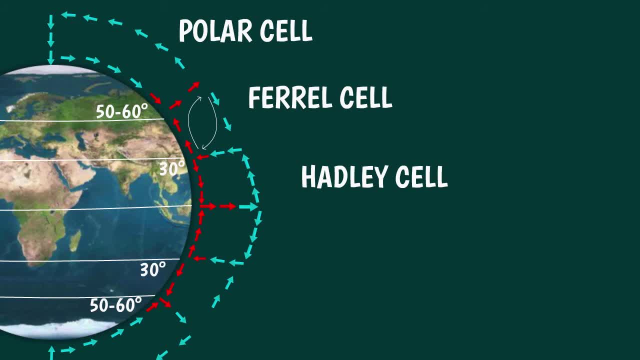 The reason for this is that the air in the Hadley cell and in the polar cell moves due to temperature differences, while the ferrule cell owes its existence to the presence of the other two cells. The overall effect of the three cells and of atmospheric circulation. 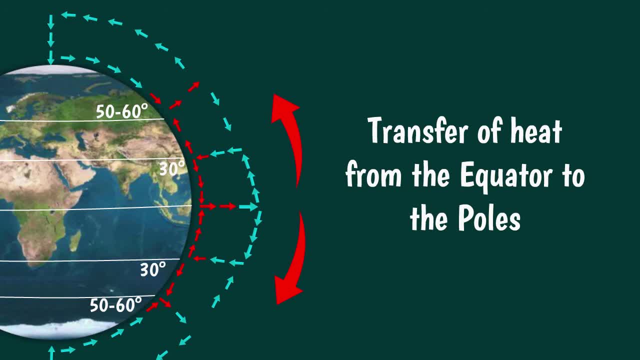 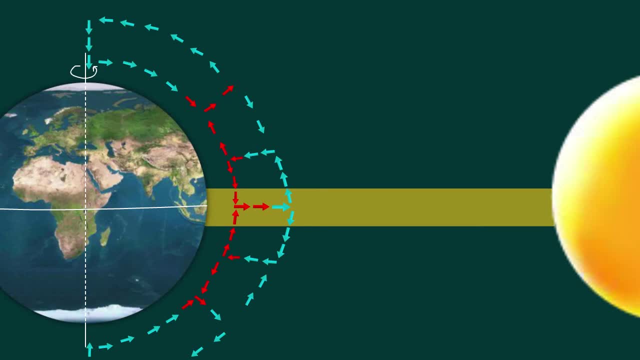 is to redistribute heat between the equator and the poles, preventing the equator from getting hotter and hotter and the poles from getting colder and colder. It should be noted that the exact position of the cells varies with the seasons. For example, in June. 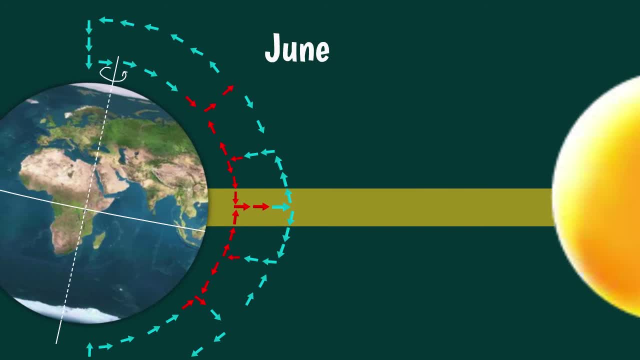 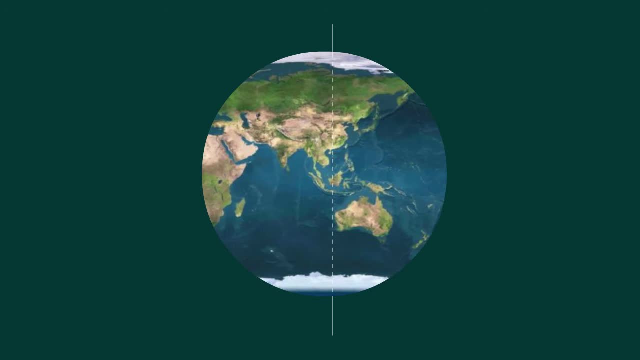 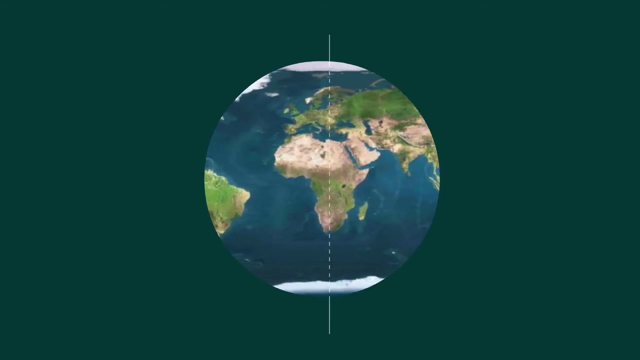 it is summer. in the northern hemisphere, everything moves a few degrees to the north, while in December the cells move to the south. In addition, we have not yet taken into consideration the fact that the earth rotates on its axis. This strongly impacts atmospheric circulation due to a phenomenon called Coriolis effect. Let's see what that is. 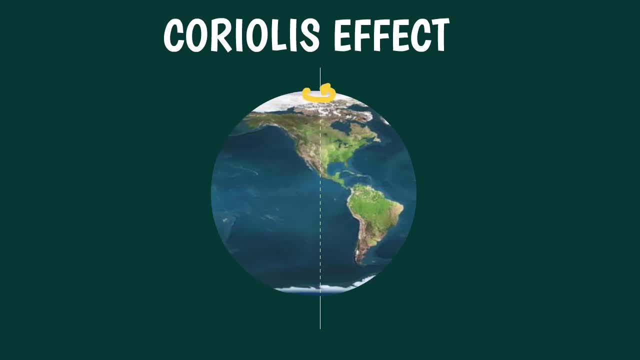 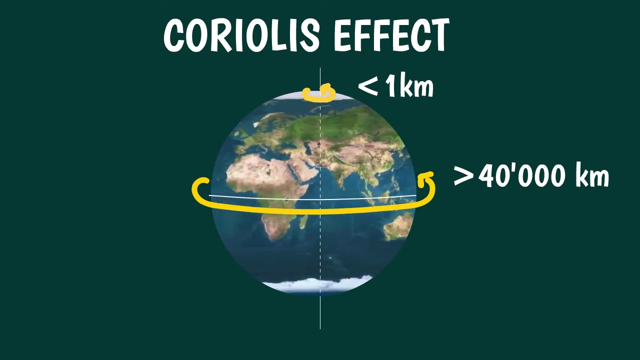 You probably know that every 24 hours, the earth completes a rotation on its axis. However, a locality near the poles has only a very small loop to go to make a full circle, But a locality at the equator has to travel more than 40,000 kilometers to get back to the same spot. 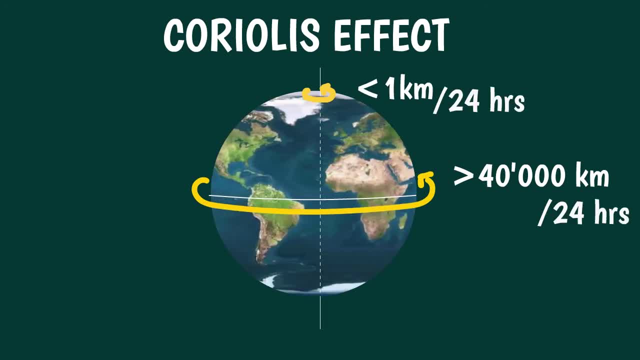 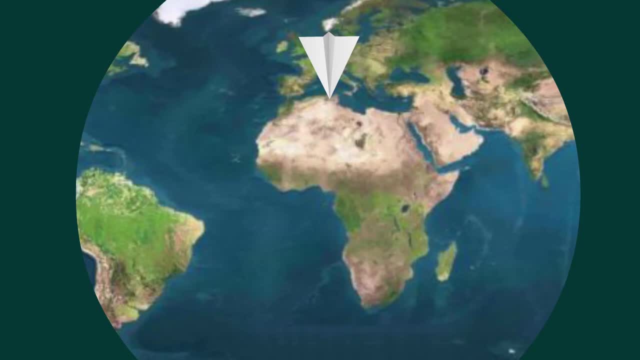 So since all the points on the surface complete the loop in 24 hours, those near the equator must necessarily rotate at a much greater speed than those near the poles. Now imagine that you throw a paper plane capable of flying thousands of kilometers and that from Europe, you throw it due. 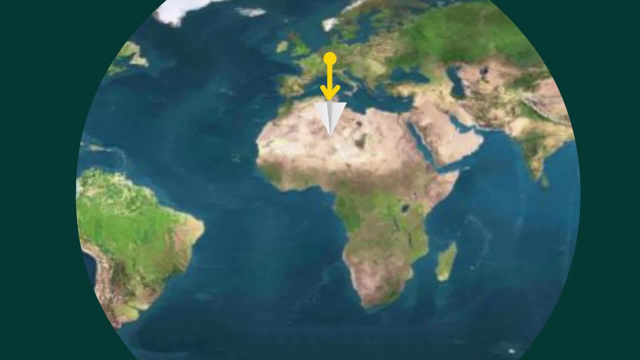 to the fact that it is a very small plane. Normally you would expect the plane to land in a location that is directly to the south, that is, at the same longitude, Except that, as we have just seen, the localities near the equator turn much faster than the starting point. 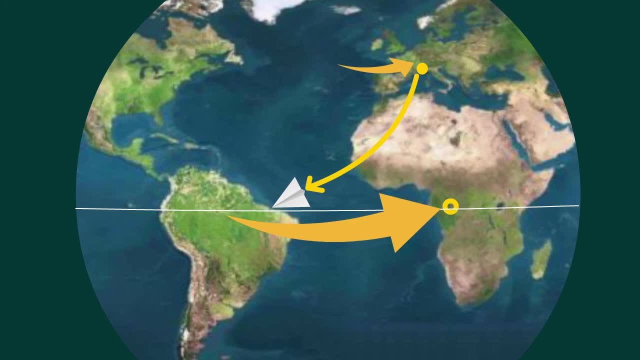 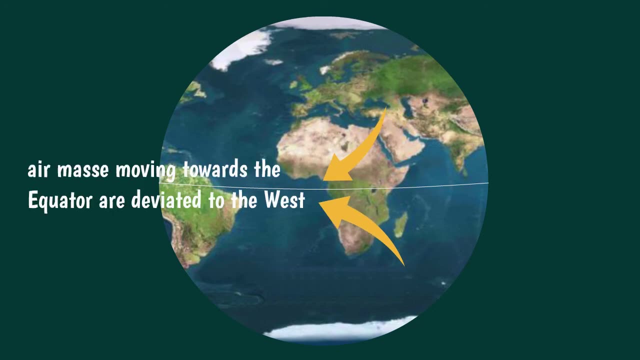 in Central Europe. So your plane will end up falling well to the west of the starting point. The same thing happens with air masses: When they move towards the equator, they are deviated towards the west And, on the contrary, when they travel towards the poles, 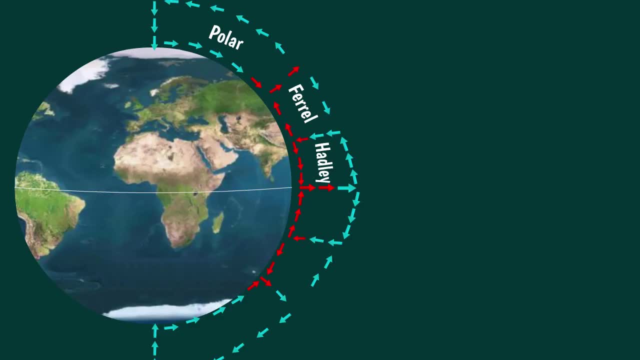 they turn towards the east. So if you go back to ourselves, the Coriolis effect causes air moving from areas at 30 degrees latitude towards the equator to turn west. In the regions around the equator we expect to have winds which blow from the northeast to the southwest. in the northern 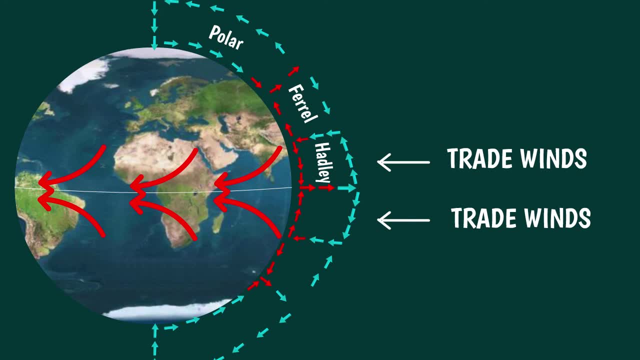 hemisphere and from the southeast to the northwest. in the southern hemisphere, These winds are called the trade winds. On the contrary, at mid-latitudes, say, between 30 and 50 degrees, the air that moves towards the poles is deviated from the west to the east. For this reason, 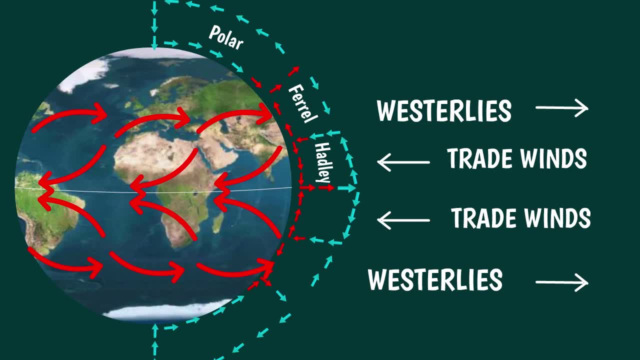 if you live in Central Europe, you will observe that most of the time the wind blows from the west. In the next video, we will discuss the effect of atmospheric circulation on the planet's climate and, in particular, we will see how this leads to the formation of different climatic zones. 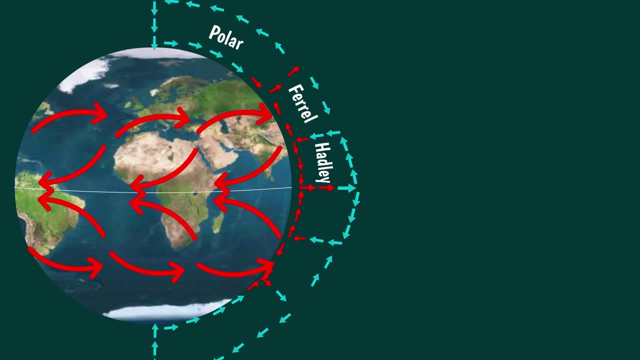 In the meantime, thank you for subscribing to our channel and see you soon.